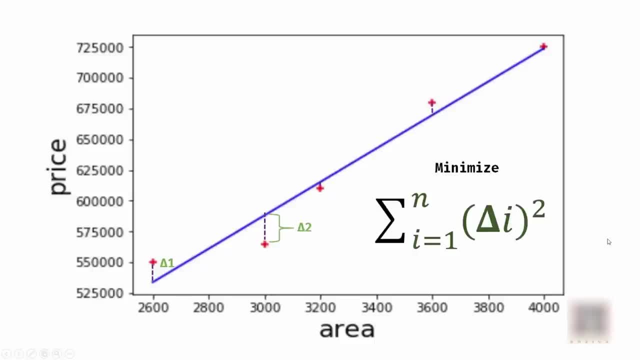 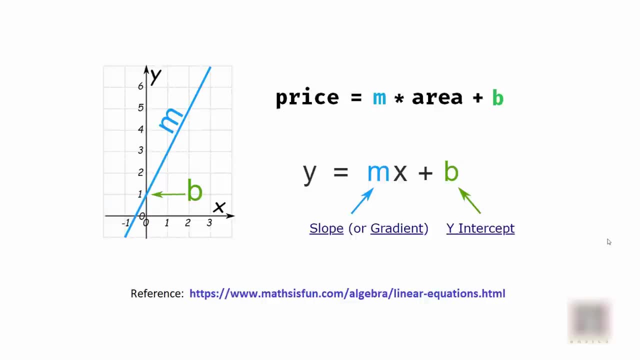 Now, if you remember from your algebra class- you had the answer to this question class during your school days- then you you have probably learned the linear equations, which looks like Y is equal to MX plus B, where M is a slope or gradient and B is an intercept. in our case, the slope is M here, but the Y is price, and 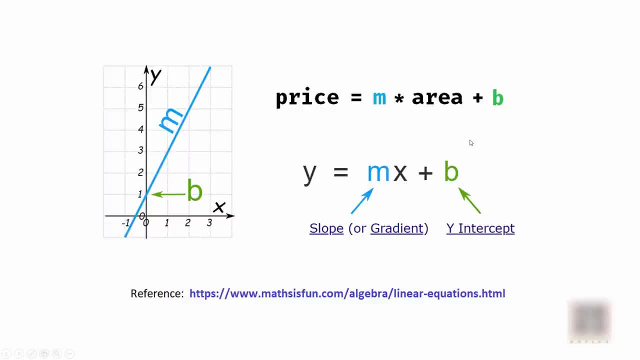 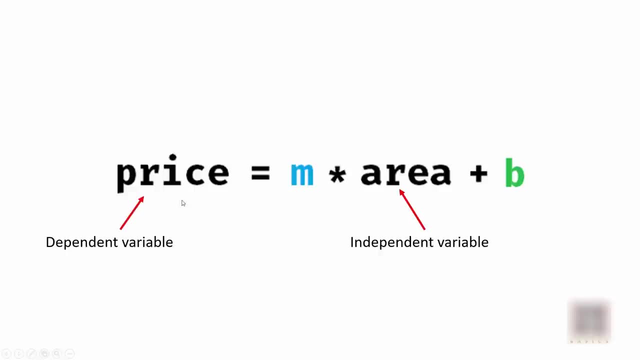 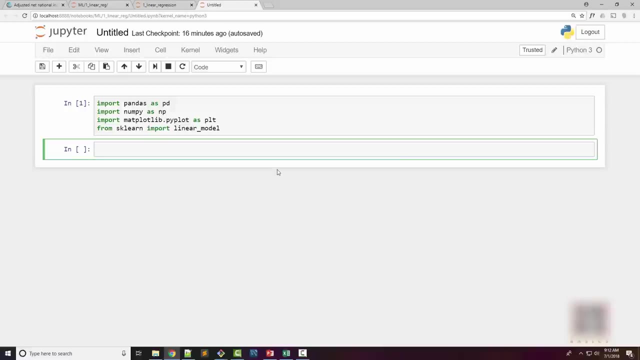 an X variable is area. area is called an independent variable, whereas price is called a dependent variable, because we are calculating price based on this area. now we are going to write Python code for doing home price predictions here. I have launched my Jupyter notebook and I have imported some useful libraries. the 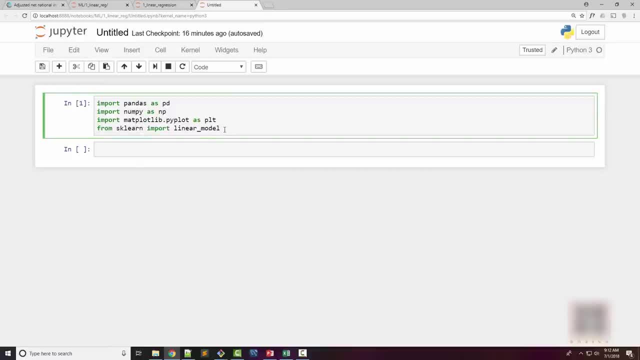 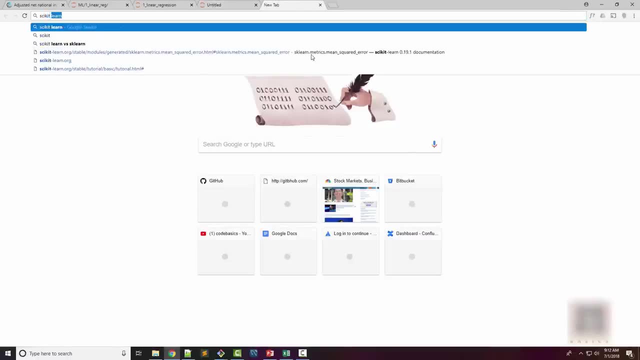 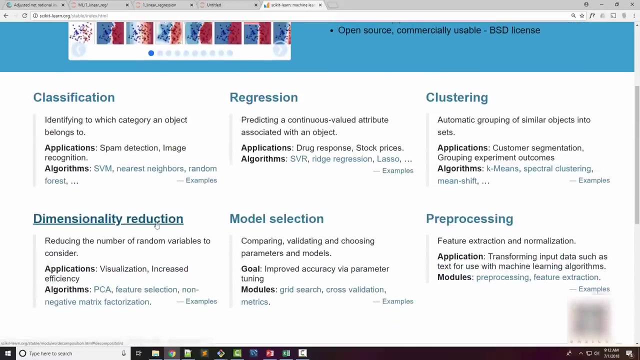 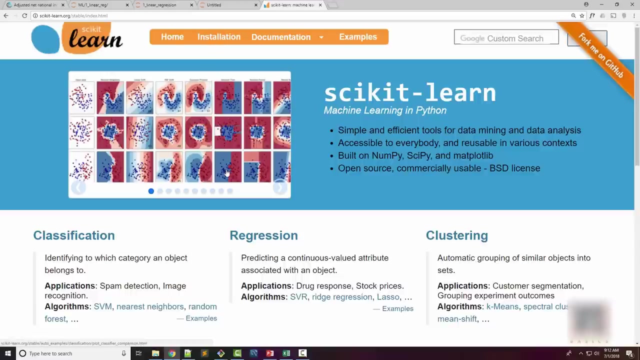 most important library here is from sklearn import linear model, so sklearn is the library. it is also called scikit-learn, so if you google it, you will find that this is the library we are using and it comes with anaconda installation. so once you have installed anaconda, you should have this. 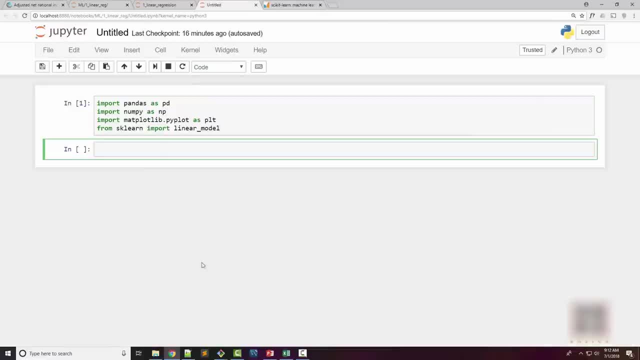 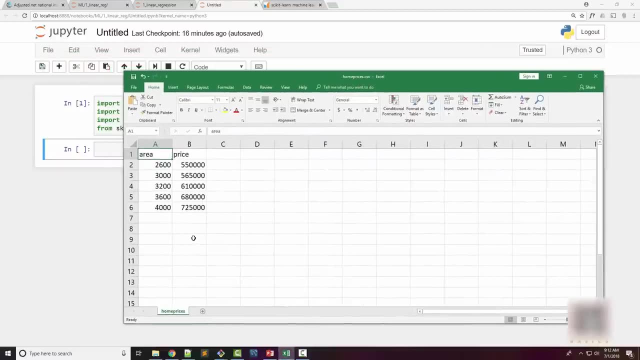 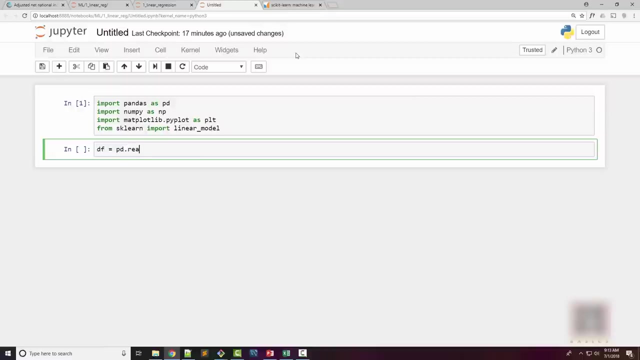 library available for import. I have the prices available in the description of this video. if you have any questions, please feel free to contact me at Dc. Dc file address in the description of this video. so the first thing I'm going to do is load this. prices in pandas data frame, PD, dot, read. 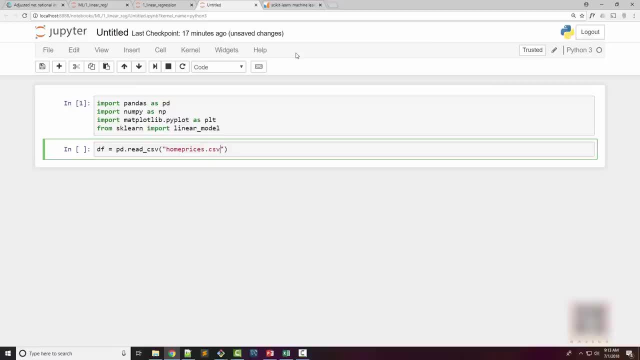 CSV. name of the file is home prices dot CSV, and I have the data frame now. if you don't know about pandas and data frame, I recommend you watching my tutorials on pandas, because pandas is going to be extremely useful for your courses. so, as you can see, I am using cyberspace to create this file. so if you don't know about pandas and data frame, I recommend you watching my tutorials on pandas, because pandas is going to be extremely useful for you all the time. so if you are interested in this, let me know by clicking on the link in the description below. 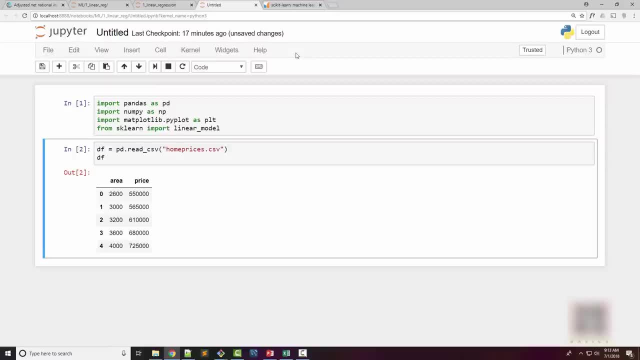 uh, in your machine learning journey, once i have a data frame, uh, next thing that i'm going to do is, uh, plot a scatter plot just to get an idea on the distribution of my data. point. okay, and you all know, uh, if you have used jupyter notebook before, is that you have to use a matplotlib. 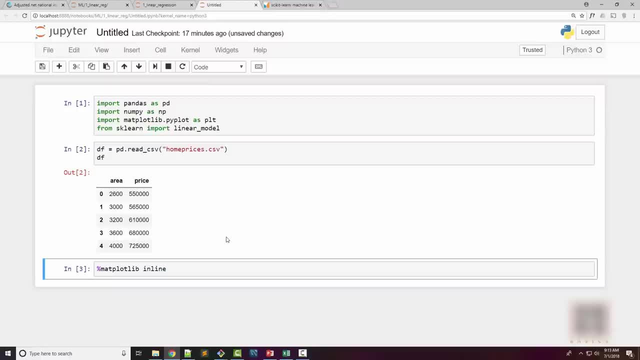 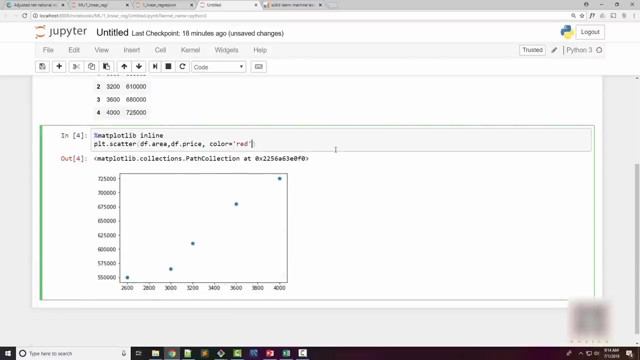 inline magic, uh, in order to draw the plots, and first i'm going to uh, plot dot scatter, so i'm going to plot area versus price. okay, now i'll make some modification and i will set color to be red marker to be plus. i'm just making some modifications and i will set color to be red marker to be plus. i'm just making some. 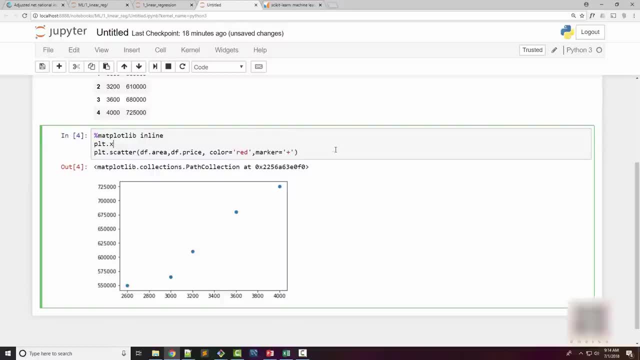 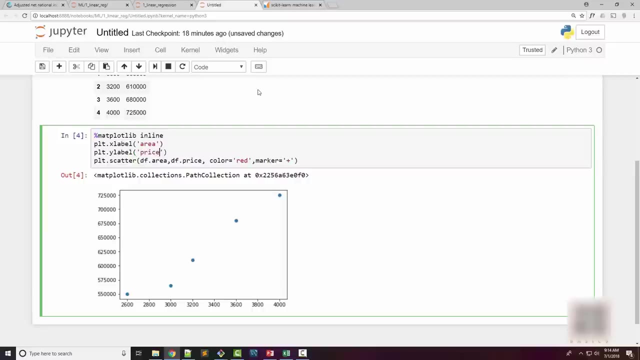 making my chart little fancy and then also setting x and y label, because you can see that x and y labels are not available right now. so the x label would be area in square fit and y label is the price in us dollar. okay, so this is square fit area and us dollar price, all right, so once i 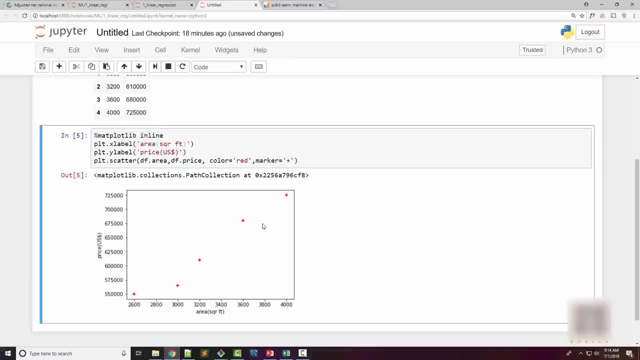 look at the chart. i'm going to set the color to be red, marker to be plus. i'm just making some modifications. and i will set color to be red, marker to be plus. i'm just making some modifications at this plot. i get an idea that the distribution is suitable for a linear regression model and 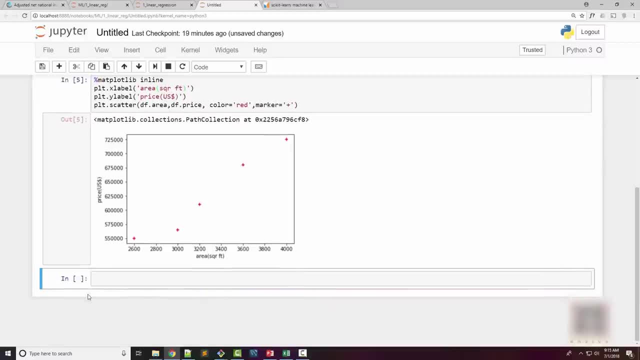 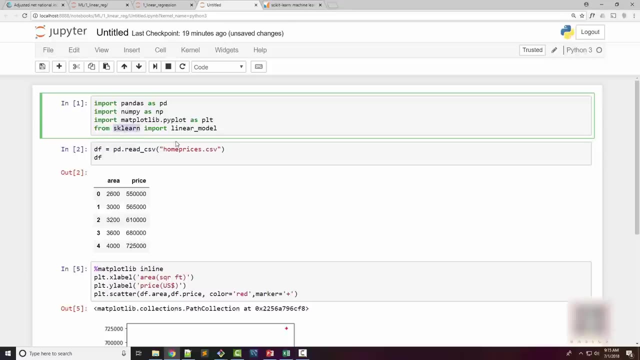 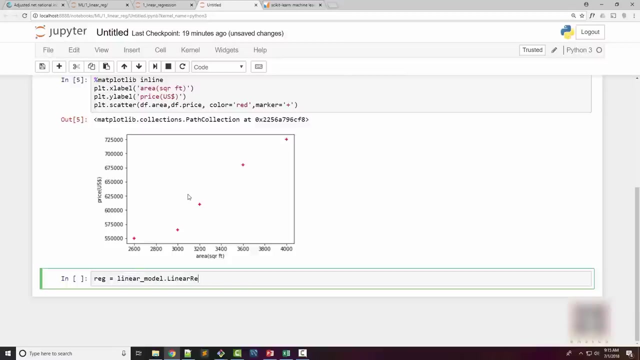 hence i will now go ahead and use the linear regression. okay, so first you need to create a linear regression object so you can see that from sk learn python module i have already imported linear model and here linear regression. so i will create an object for linear regression and then i will fit my 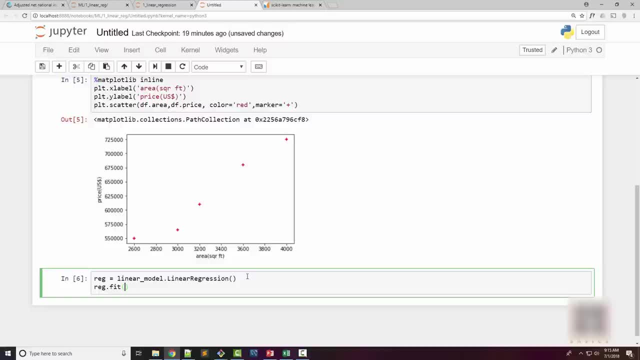 data. so fitting the data means you are training the linear regression model using the available data points. okay. now the first argument has to be like a 2d array, so you can supply your data frame here. so i am going to supply a data frame which only contains area, okay. and the second. 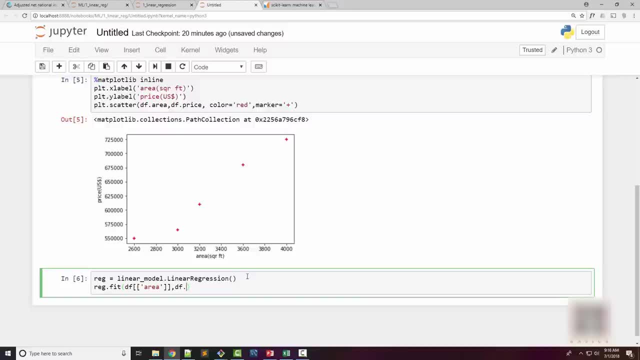 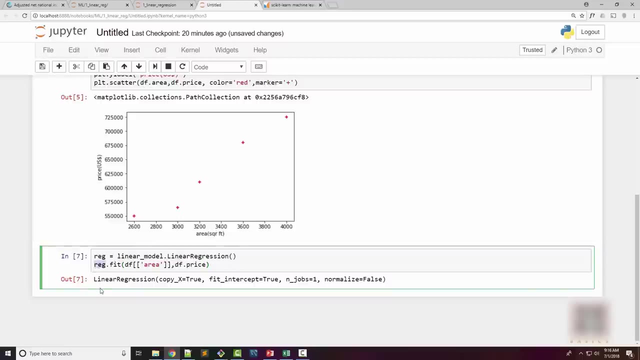 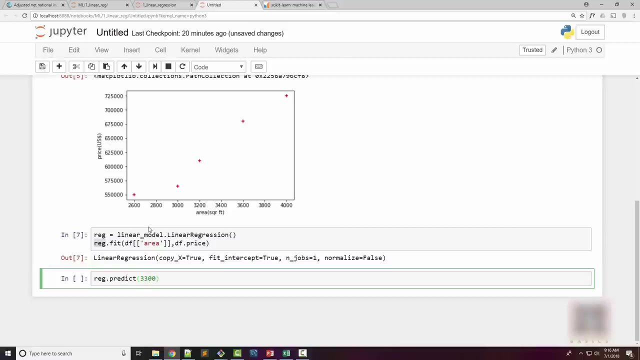 argument would be your y-axis on your plot, which is your price. so when i execute this, it worked okay without any error, which means now this linear regression model is ready to predict the prices. so let's do our prediction. so what we wanted to predict was the price of a home whose area is 3300. 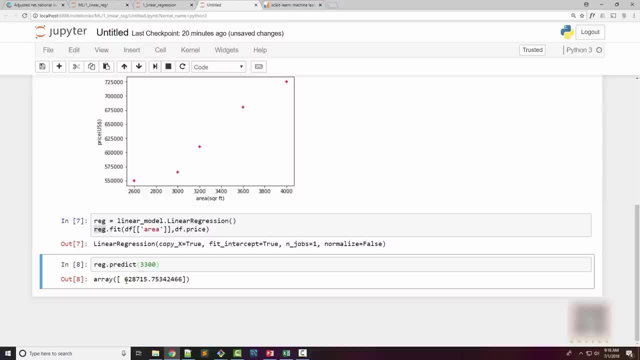 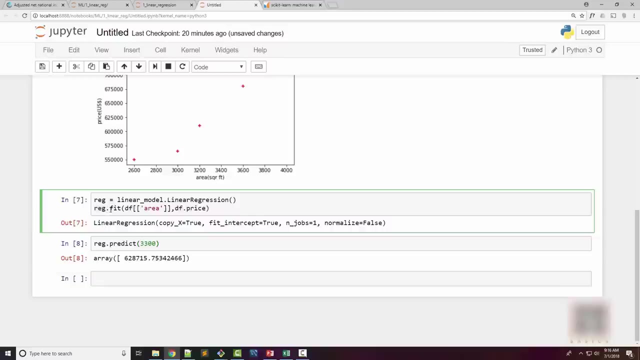 square feet and you can see that it predicted this price. now you might be wondering why it came up with this price, so let's look at some of the internal details. so when i train my regression linear regression object, i will be able to see that the price of the home is 3300 square feet. 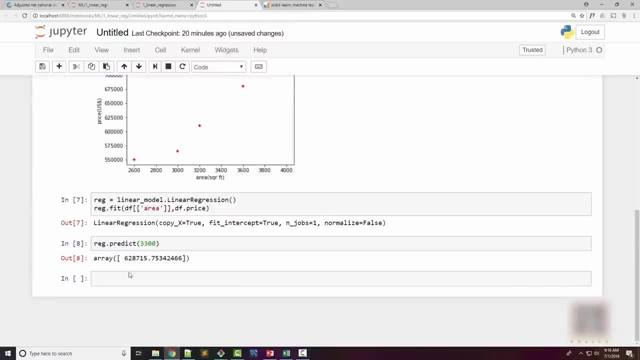 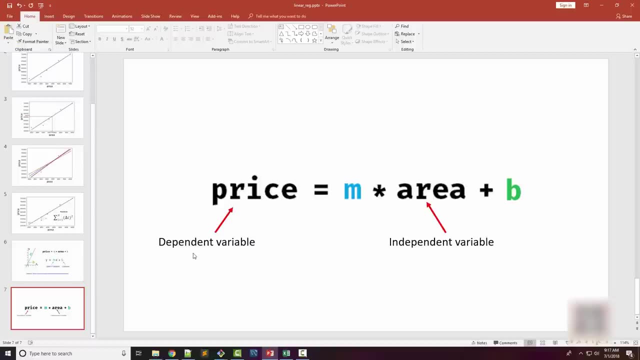 and the price of the house has a value of 12 대박. what it actually did was it calculated the value of the roof off the brick. so on a straight Sequence, we do theCollection. now conclusions are the values of f and b. Oops pretends the price of the house is about 324- killsback. 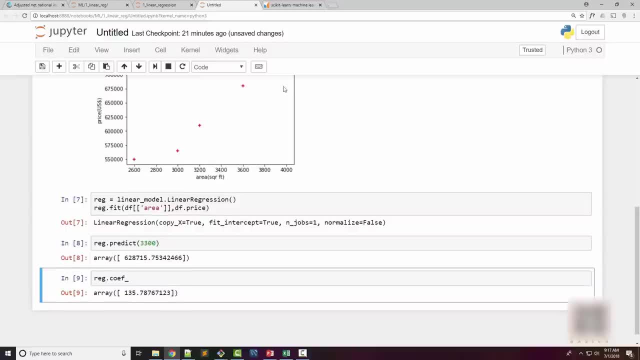 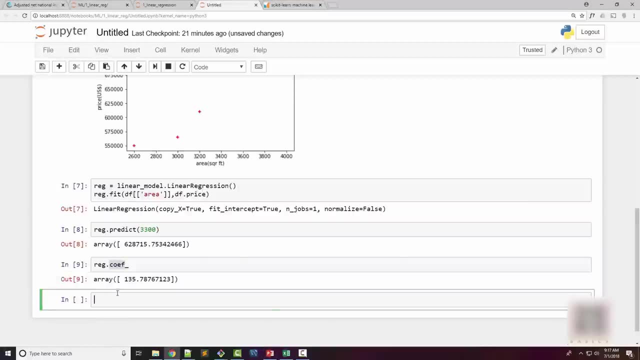 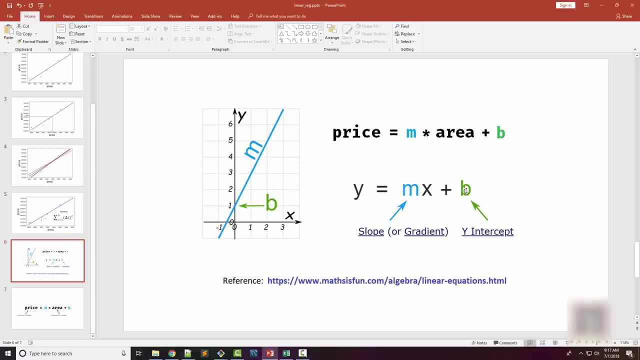 because, again, that is not surprising regcoef- it will show the value of coefficient, which is this m, and when you do intercept, this is showing you the, the value for this b. okay, so now the equation for price is m into area plus b. okay, so now we have m, area and b, so let's see what value it gives. 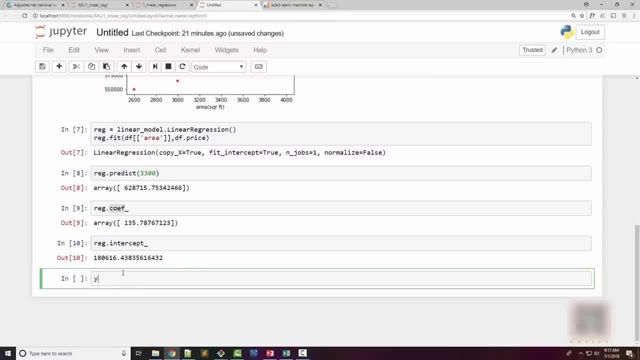 so y is equal to m into X plus B. okay, and here M is this number. so let me just copy it into X. X is the area that you want to predict. so area you want to predict is 3300 and your intercept is this: okay, so when you execute this, you get this value. so now you know how it was able to predict this. 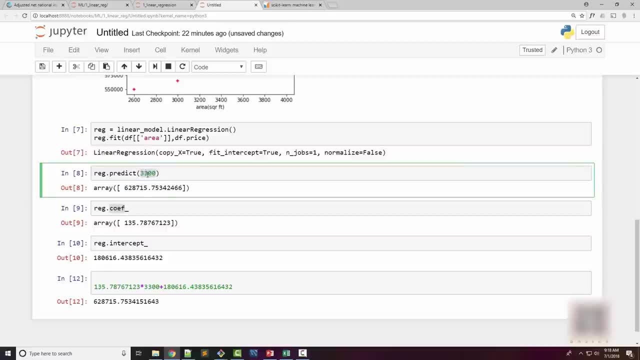 value right here, okay, similarly, if you change this to the second value that we wanted to predict was the 5000 square feet, so for 5000, you can just do this and you get this value right here. so this is very amazing. now you have a model which you can use to predict your home prices. uh, you might have. 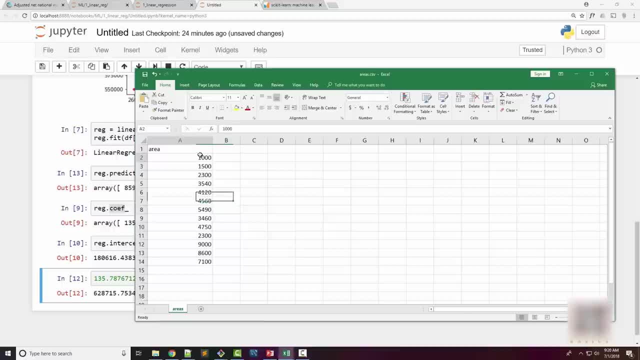 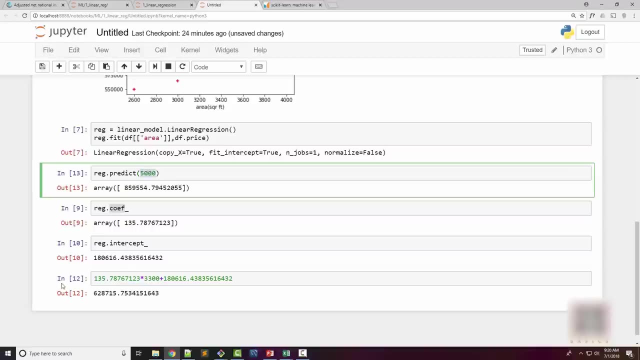 a CSV file like this, where you have list of prices, a list of areas available and you want to predict, uh, the prices for these homes. right until now, what we did is we were individually giving them on the area and we are predicting the prices. so what I want to do now is generate another CSV file. 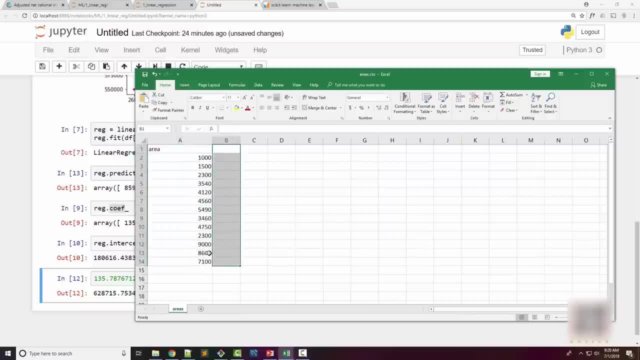 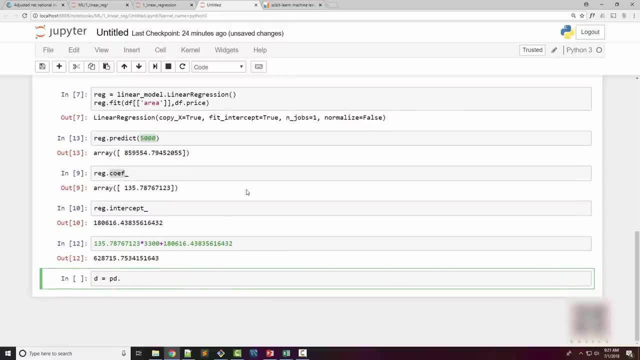 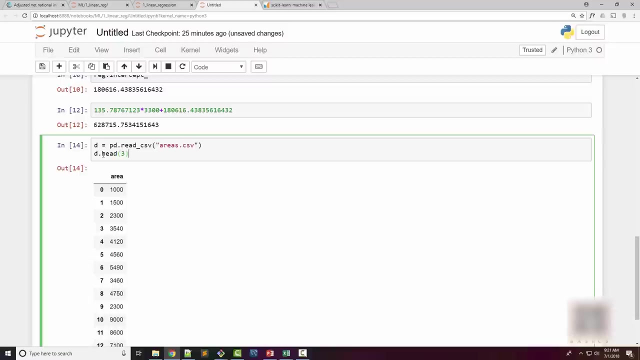 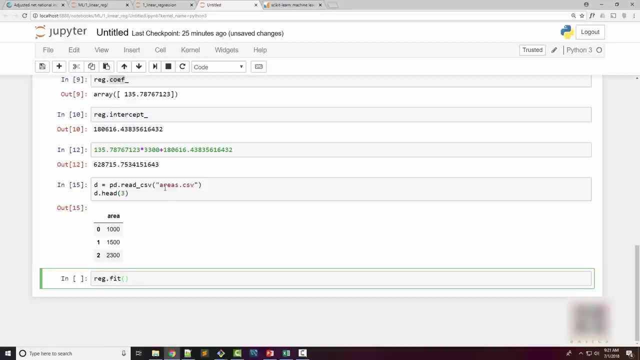 of areas and their corresponding prediction on prices. so for this I will create a data frame first using read CSV. so here first I created a data frame. I have list of areas available. now I will use regression model to actually predict the prices. okay, so I'll just supply D here and that will return me the prices. 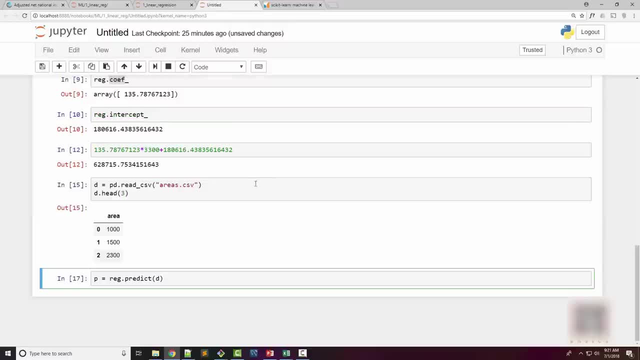 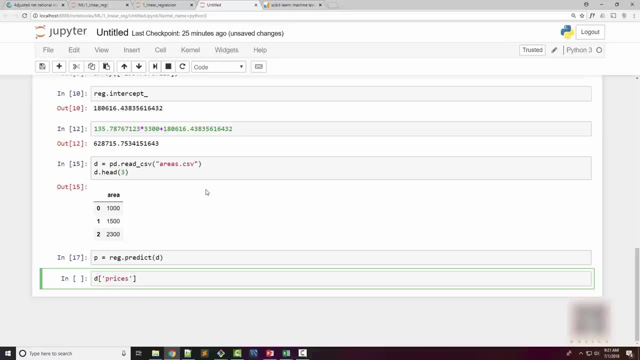 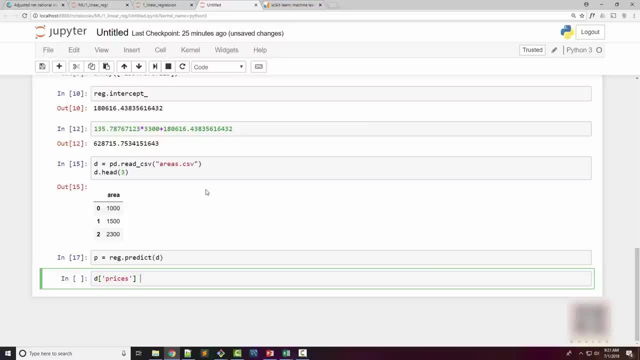 in your original data frame you can create a new. in your original data frame you can create a new column. so when you do like this, it column. so when you do like this, it column. so when you do like this, it will create a new column in your data frame. 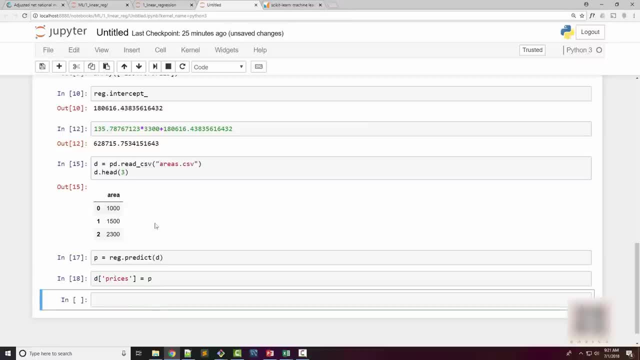 will create a new column in your data frame. will create a new column in your data frame and you can assign P here: okay, and. and you can assign P here: okay, and. and you can assign P here: okay, and now, when you print your data frame, you can. 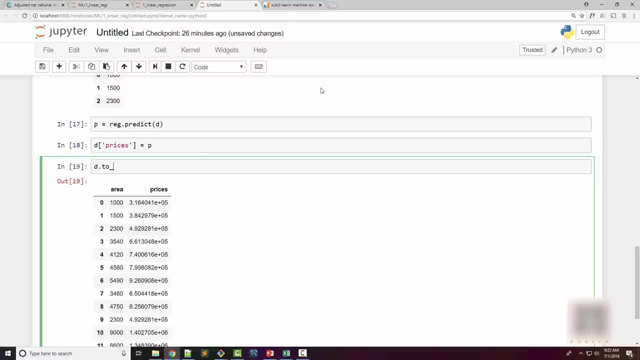 now when you print your data frame, you can. now, when you print your data frame, you can see the prices are available and then see the prices are available and then see the prices are available, and then you can just use to CSV method to export. you can just use to CSV method to export. 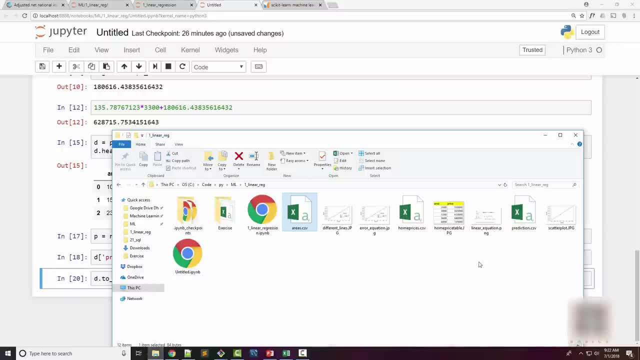 you can just use to CSV method to export the value to prediction dot CSV. so if I the value to prediction dot CSV, so if I the value to prediction dot CSV, so if I open my prediction dot CSV, you will now open my prediction dot CSV. you will now 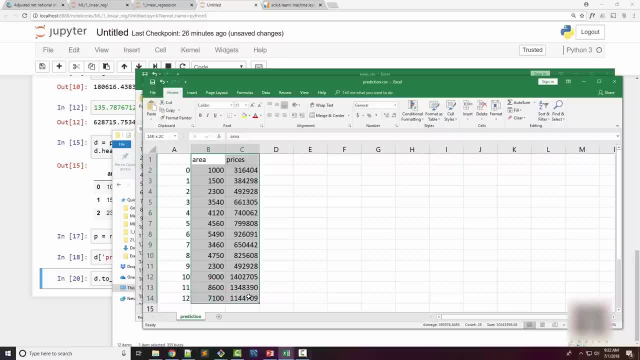 open my prediction, dot. CSV. you will now find that I have area and prices. it find that I have area and prices. it find that I have area and prices. it imported. it exported actually the index imported. it exported actually the index imported. it exported actually the index as well. and if you don't want to do that, 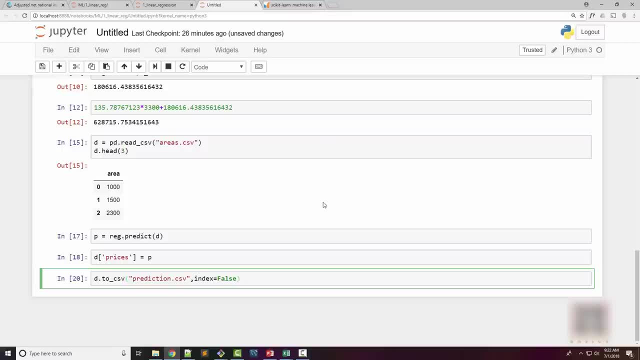 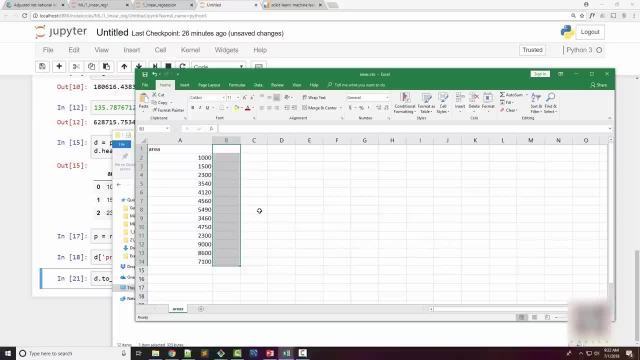 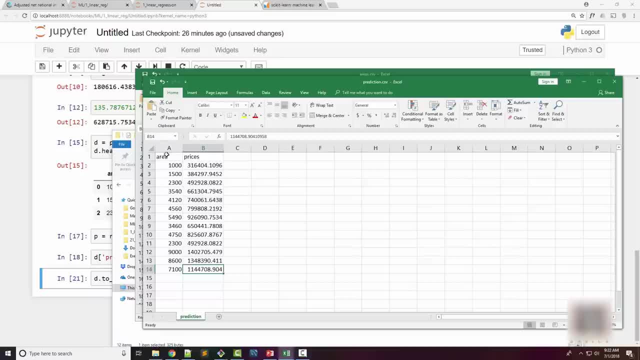 won't find the index. it will be just won't find the index. it will be just area and prices as you can see here: okay. area and prices as you can see here: okay. area and prices as you can see here: okay. so once you have this model built in, 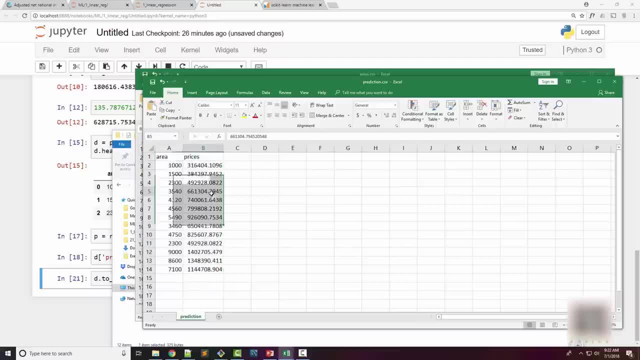 so once you have this model built in. so once you have this model built in, you can apply this model on a huge CSV. you can apply this model on a huge CSV. you can apply this model on a huge CSV file and come up with a list of. 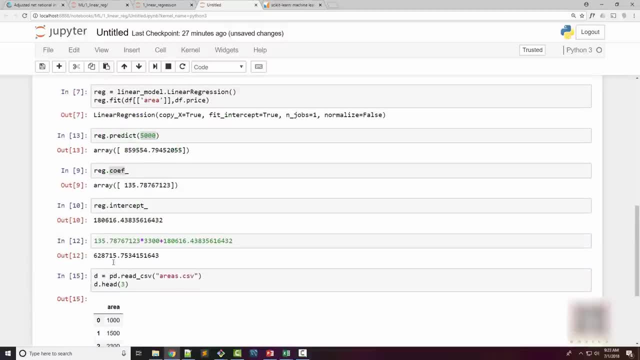 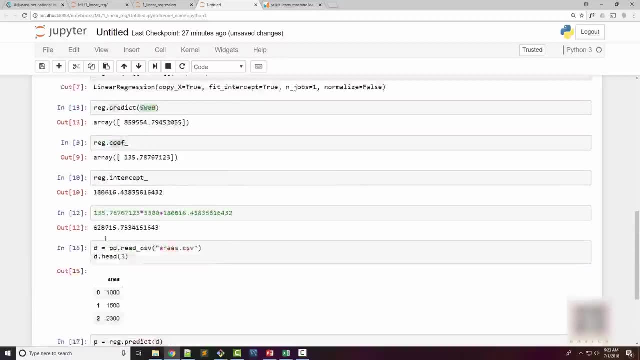 file and come up with a list of file and come up with a list of predictions- now going back to our predictions, now going back to our predictions, now going back to our original example. so let me original example, so let me original example. so let me go back again here and read my original prices. 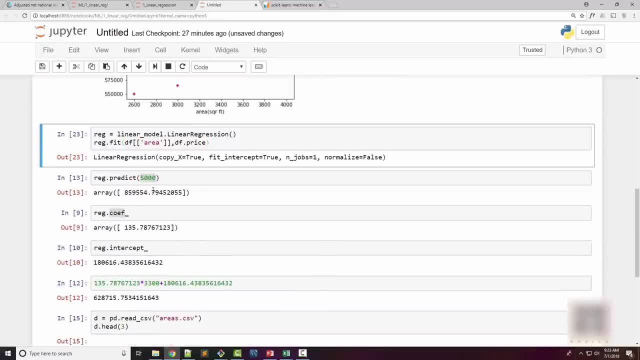 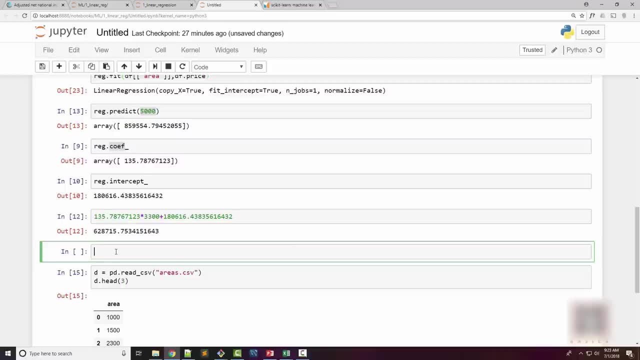 go back again here and read my original prices. go back again here and read my original prices and do a fitting on that. what I and do a fitting on that, what I and do a fitting on that. what I want to show you is how does my linear 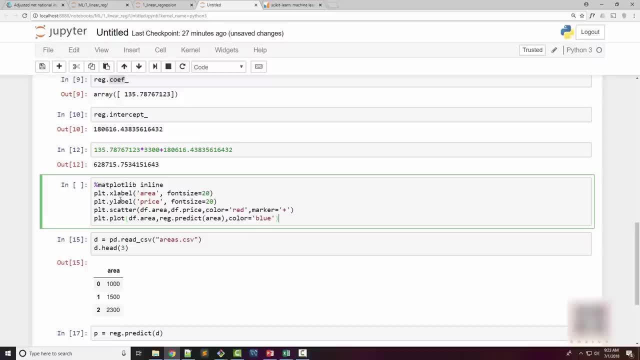 want to show you is: how does my linear want to show you is: how does my linear equation line look okay, and for that I'm equation line look okay, and for that I'm equation line look okay, and for that I'm again plotting a scatterplot and along. 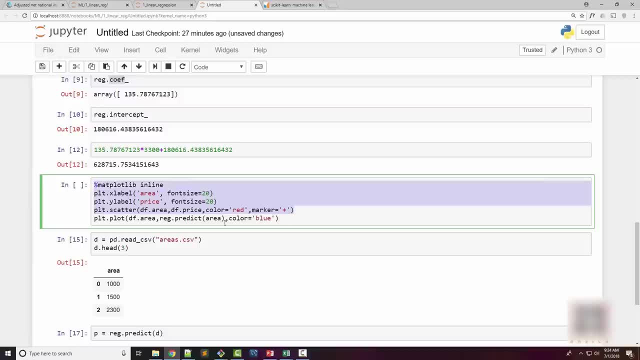 again plotting a scatterplot and along again plotting a scatterplot and along with the scatterplot. so this much line with the scatterplot, so this much line with the scatterplot, so this much line of code will just applaud of code will just applaud the scatter plot. and I have added one more line where I'm using data frames. 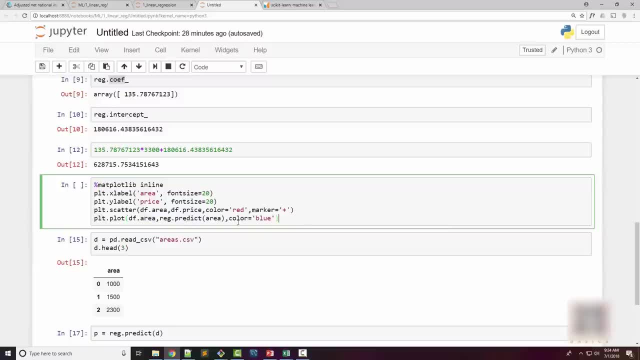 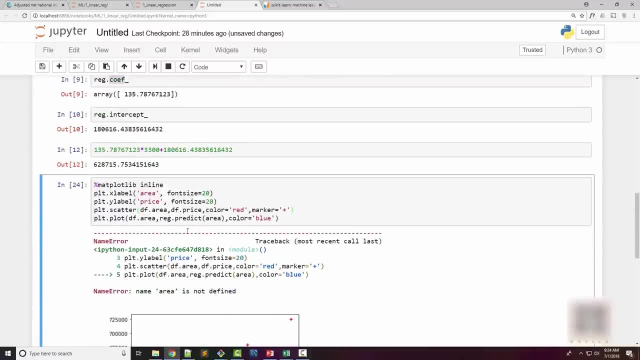 area and I am predicting the prices and plotting them on the Y chart. so let's see what happened here. so DF dot area is not defined, so that has to be the F dot area here. so let's go step by step. so here I have my scatter plot and what I'm 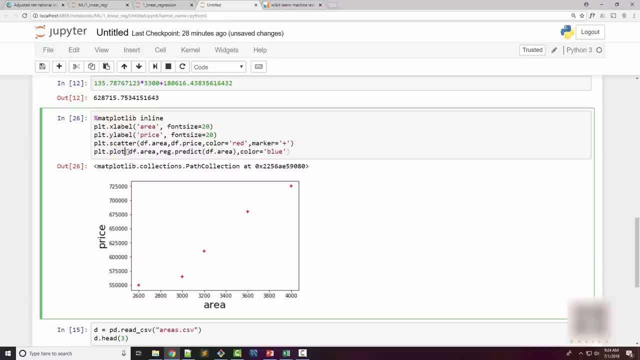 doing is PLT dot plot. on my x-axis I want the F dot area and on my y-axis I want to. I want to predict area like this. okay, so it shows the visual representation of my linear equation here. all right, so that's all I had for this tutorial. I have an exercise for you. 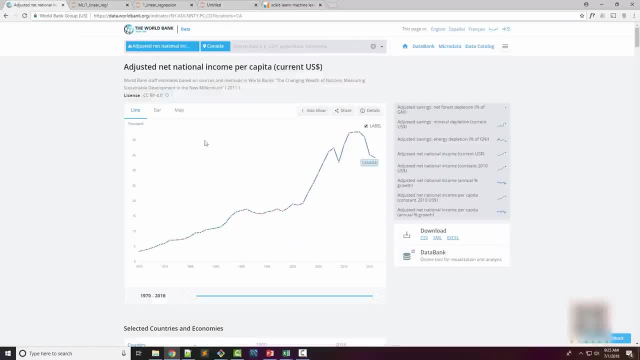 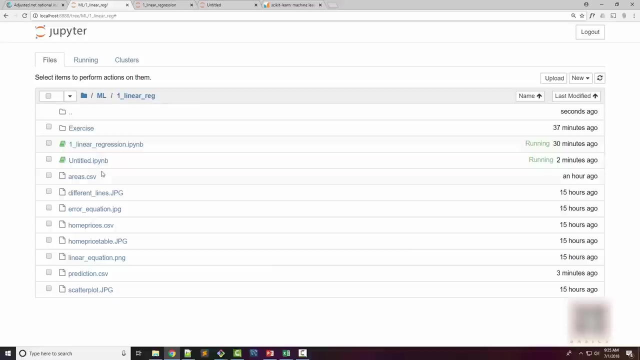 guys, what you want to do is, given Canada's adjusted net national income per capita, you want to predict the net income in year 2020. I have provided a CSV file in the exercise folder. so if you go to github and download my notebook- and I have, by the way, the link of Jupiter notebook- 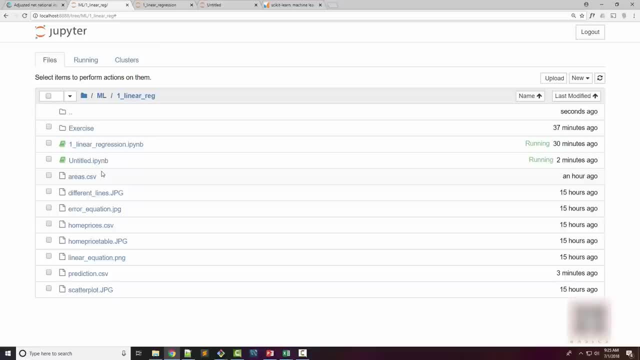 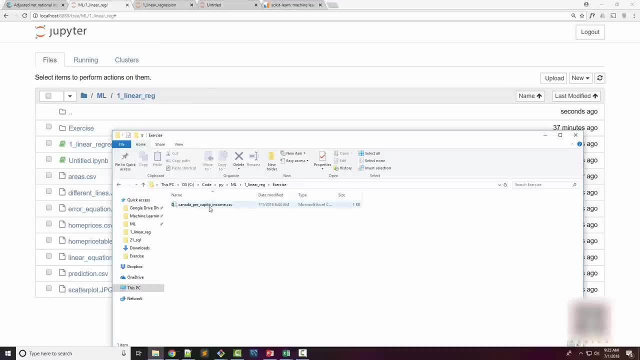 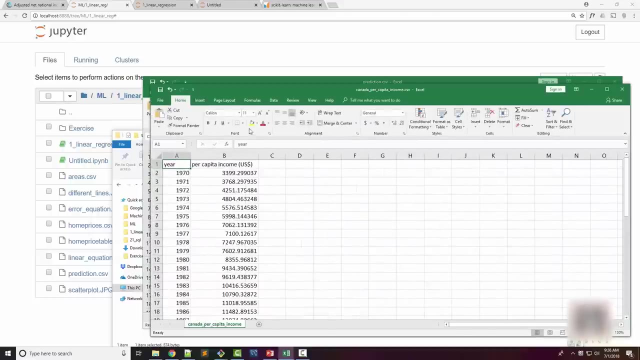 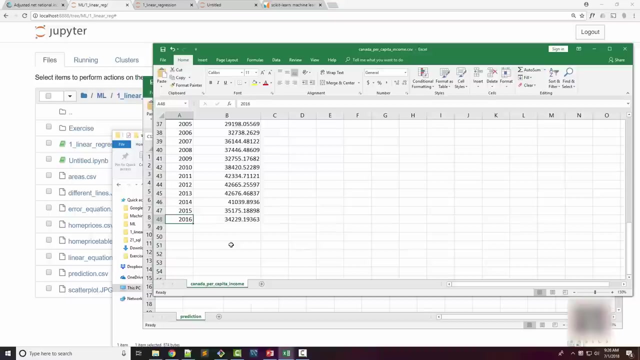 available in the video description below. so download the notebook, study it first and then download the exercise folder. in the exercise folder you will find this so that you can use it for the year 1970 to 2016, and your job is to find out the 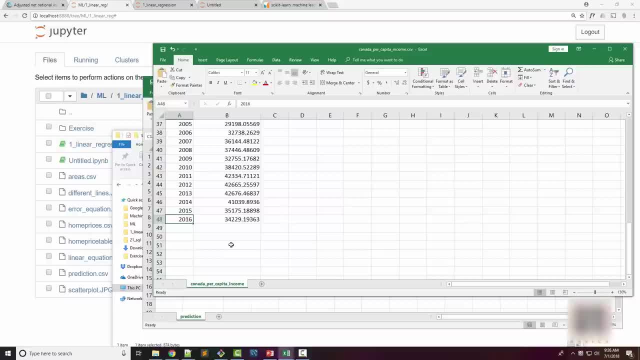 predicted income in year 2020. I highly recommend that you do the exercise, because just by watching the video, you are not probably going to learn that much. I mean, you learn something, but it's not very effective, so it's it's better that you do some practice as well, as we go through these tutorials, and I'll make sure I provide a simple exercise in this video. 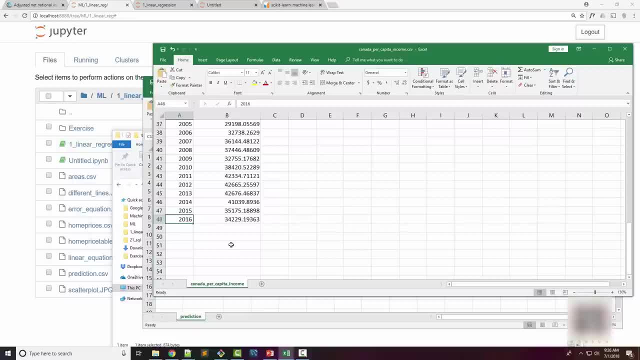 exercises at the end of every tutorial. okay, so again, just to summarize, this tutorial was all about building a simple linear regression model using one variable, and in the future we are going to cover a little more complex linear regression models. thank you, bye.